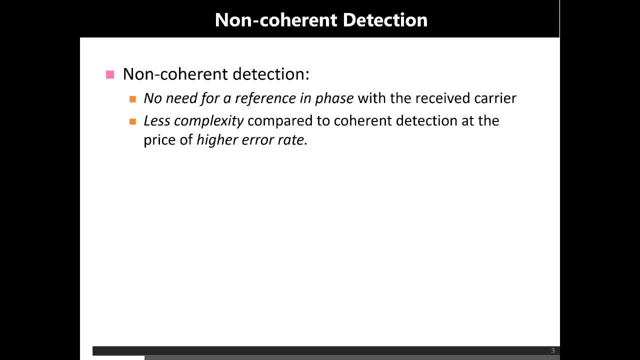 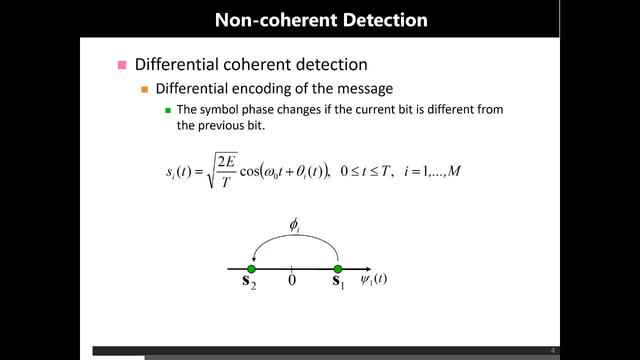 coherent detection, but definitely at a price of higher bit error rate. There are many types of non-coherent detection schemes that can be used for different types of modulation schemes, but one of the famous type of non-coherent detection is differential phase shift keying. 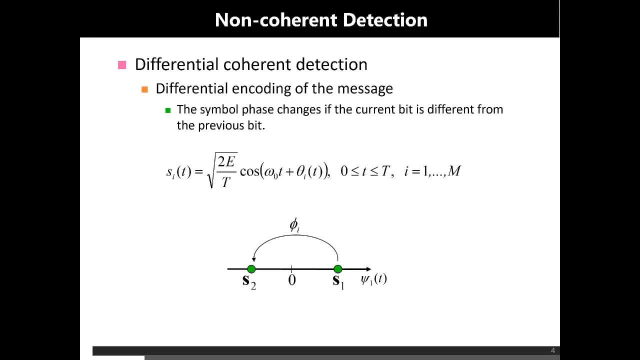 DPSK is based on a very simple and clear concept of differential encoding and what is meant by differential encoding? It means that the phase of each symbol will not depend on its absolute value, but it will depend on the previous bit. that if it is, if the current bit is the same as the previous bit. 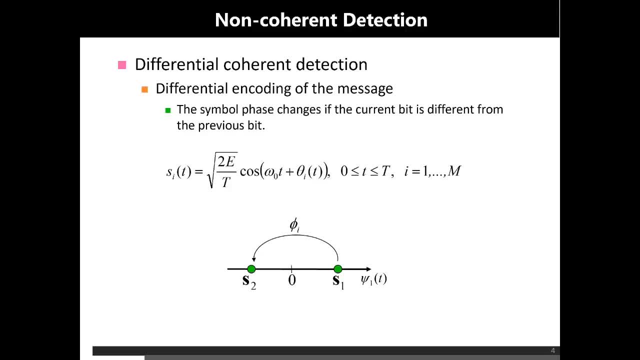 or if the current bit is different from the previous bit. So the phase assigned to each pulse will depend on, not the exact value of the current bit, but it will also depend on the previous bit and the phase will be assigned actually by means of difference between the current and the previous bit. 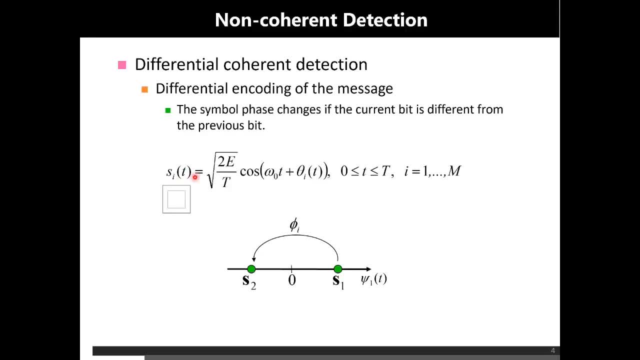 Right. So if S I of T is a transmitted pulse given by this particular expression, the information will be mounted again in the phase, as in case of phase shift keying, but in a differential manner. the phase Phi I will depend on the previous pulse. so if we are to assign a 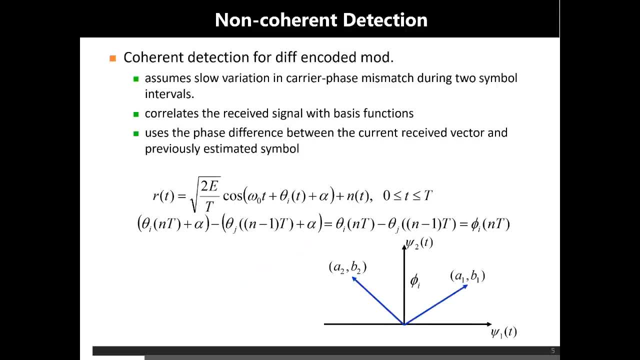 phase. for s2 it will depend on the previous pulse right. so the main basis for using differential phase shift keying is there is the assumption that the there is a very slow variation in the carrier phase mismatch during two simple intervals. because the information is now mounted on the difference in 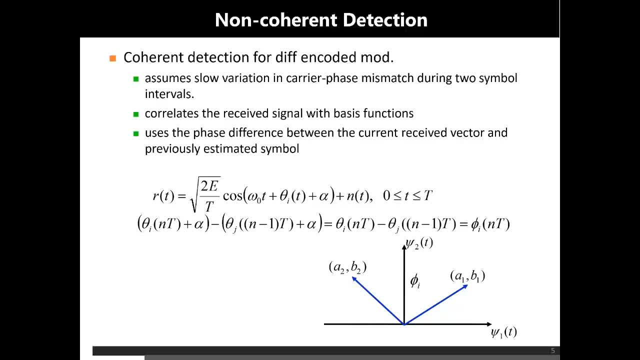 phase or the differential phase. so it is very important that the that the variations in the mismatch of phase are very slow, so that when we take difference between the phase of two consecutive symbols, that slow variation can be cancelled out right. otherwise there will be very high probability of 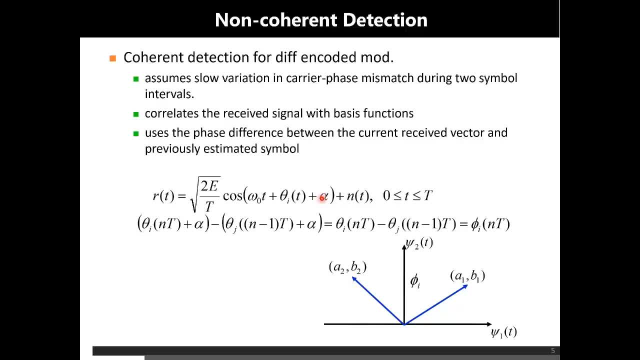 bid error. so if that slow variation is, let's say, alpha, and we have just assumed that it is not function of time because we have assumed it is a very slow variation- so if you just take the difference between the two consecutive phases, T to i and T to h, is very direct. so this is just an example which is essentially giving a 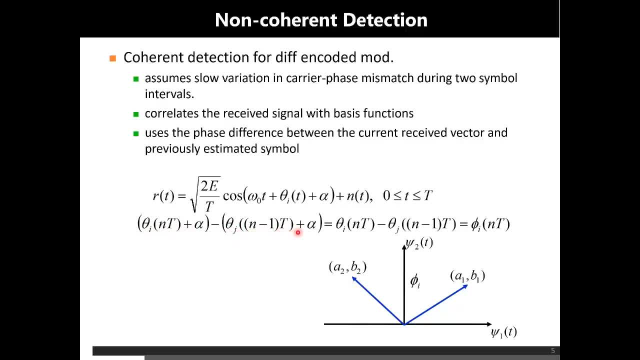 t plus alpha and theta j n minus 1 t- the previous symbol- plus alpha. so this alpha will be cancelled out and you can directly say that the information can be directly stored in the difference of phase. right, so how the receiver will be working now. the receiver will simply find out the difference. 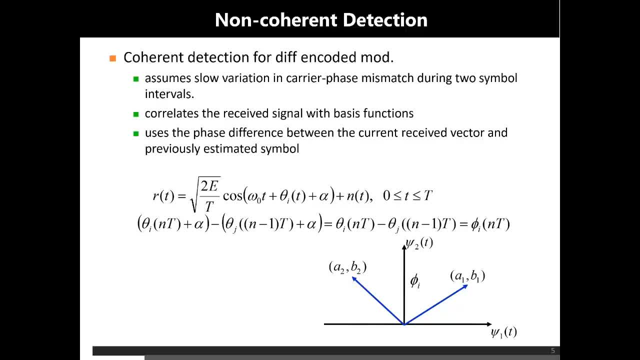 of phase of the incoming symbol and compare it with the previous symbol. so if the previous received vector was this one denoted by a1, b1, and the current received vector is given by this a2, b2, so it will simply find out the difference between the current symbol phase and the previous symbol. 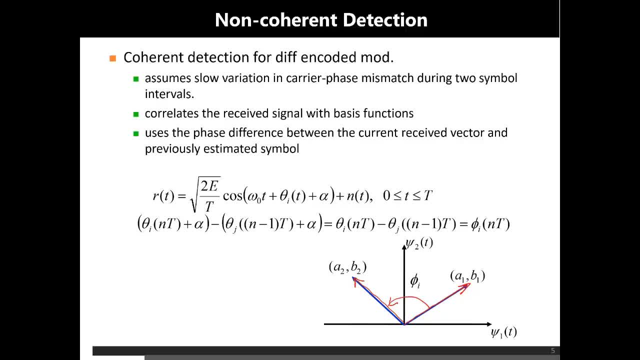 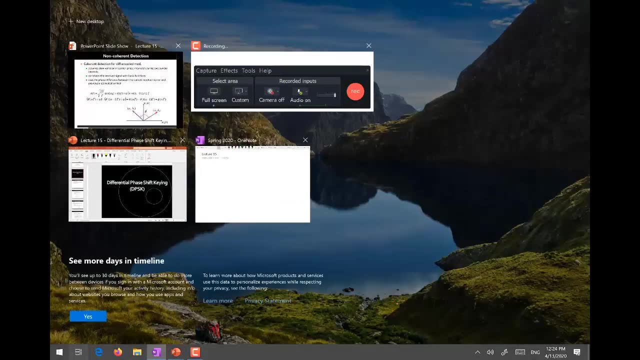 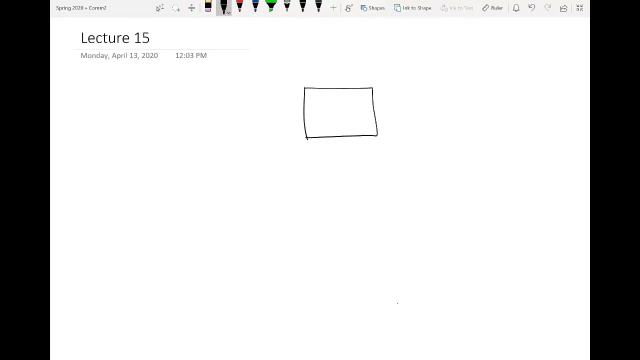 phase and use this information to detect the symbols. but you see, if we are making a receiver which is based on the difference of phase, it means we need to do some kind of encoding on the transmitter side. also, what kind of encoding is needed on the transmitter side to see the effect? just consider this particular diagram that, if we have this as 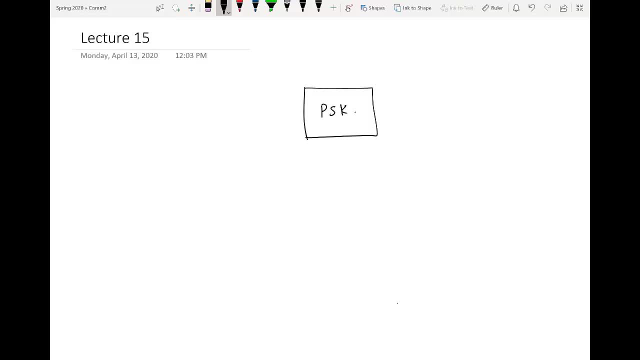 simply PSK modulator and this is the output s of T. then we need to perform some kind of additional differential encoding on the transmitter side. and what kind of transmitter differential encoding is required? it will be. it will have two options if option1 is using XOR and option 2 is using XNOR, and here we are assuming, by Binary DPSK. so for 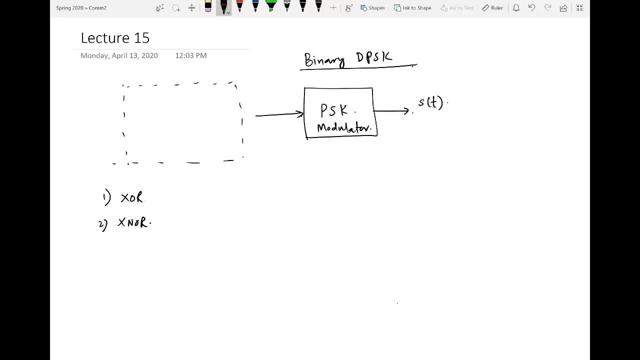 Binary DPSK. we have two options: XOR and XNOR, and how it works. for example, this is your message bits you'll printing: simply perform XOR between the current bit and the previous bit. Put a delay over here. This is the previous bit. So this encoded bit, let's say we call it CK. 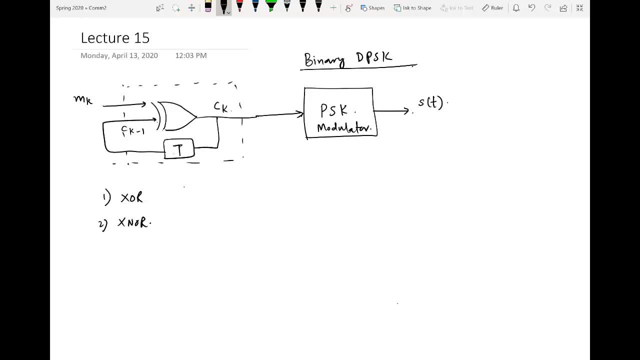 then this bit will be CK-1, so that if you are using XOR, then CK can be written as MK, XOR with CK-1.. So if you construct a simple truth table to see what is happening, then let's say: this is MK, this is CK-1 and this: 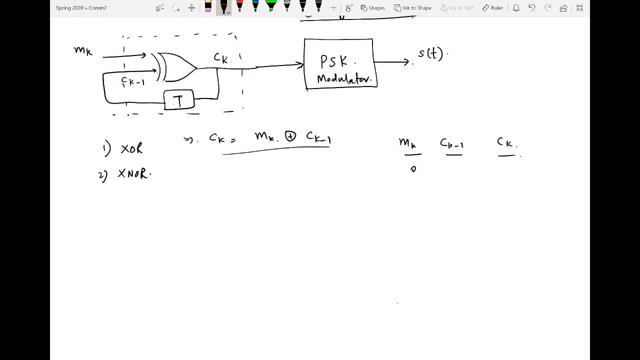 is CK, so we can have four possible combinations: 0, 0, 0, 1, 1, 0 and 1: 1.. So for 0: 0, we will have 0.. For 0: 1, we will have 0.. For 0: 1, we will have 0.. For 0: 1, we will have 0.. 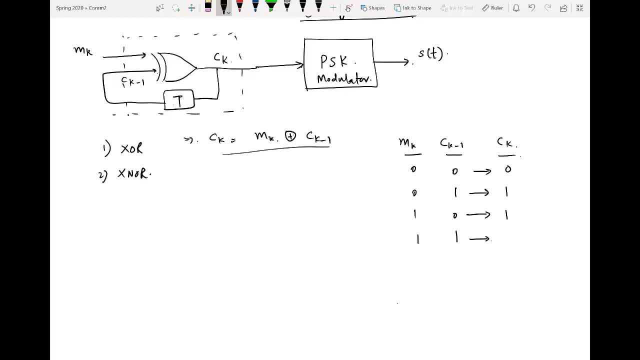 1. for 10, we will have one again. and for 1: 1 we will have 0.. What does it mean? It means that if there is a change, if there is a change in the current and the previous encoded bit, then the output will be 1, and if there is no change in. 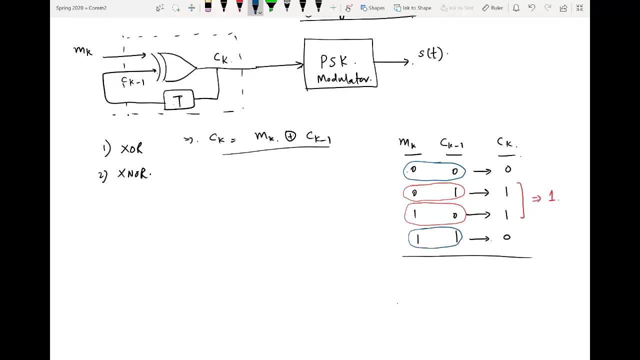 the current and previous encoded bit, like these two cases. In those two cases will have 5.. will have the bit equal to 0. so we will be only looking for a change. if there is a change in the current and previous encoded bit, then the decoded bit will be. 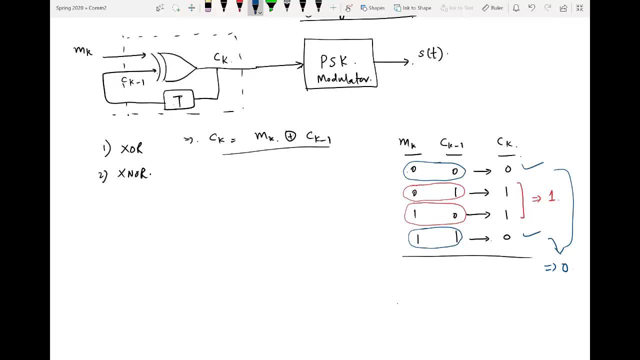 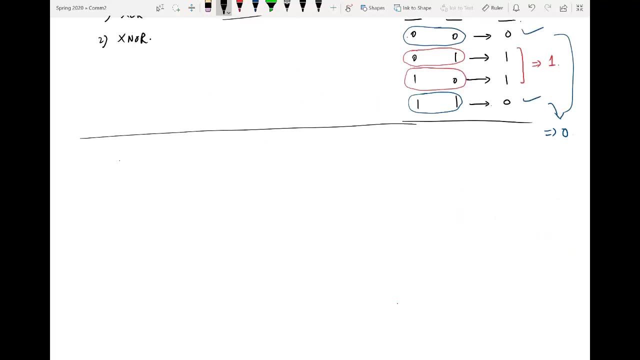 1, otherwise it will be 0, so it can be interpreted in any direction, in the forward direction or in the reverse direction. and so now let us take an example of this binary DPSK. if we say here sample index as K and the sample index is, for example, 0, 1, 2, 3, 4, 5, and these are basically message bits in the 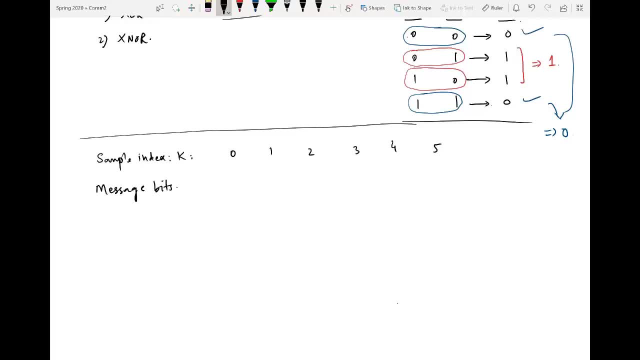 second row, denoted by MK. so the message bits start from a sample index 1 and let's say it is 0, and the message bits start from a sample index 1 and let's say they are 1, 1, 0, 1, 0, and the next one is the coded bits and we call it. 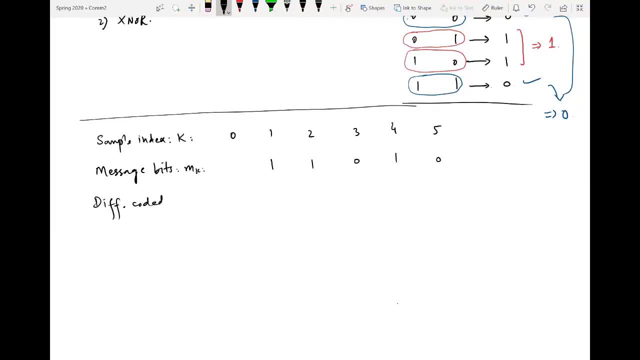 differentially coded bits, as C, K and they start from K is equal to 0, because we have to perform XOR operation for the current bit and the previous bit. so let's assume that the previous bit is 1, so Now we have to fill the other bits by performing XOR between MK and CK-1.. 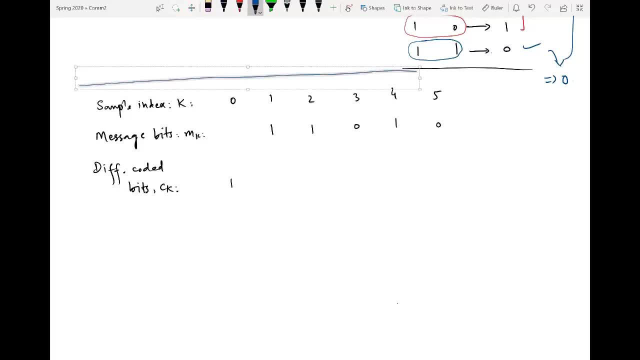 So how we will write a bit in this place. We have to perform XOR between this one, which is MK, and this is CK-1.. So by performing XOR of these two- 1, 1,- we will have 0 over here. 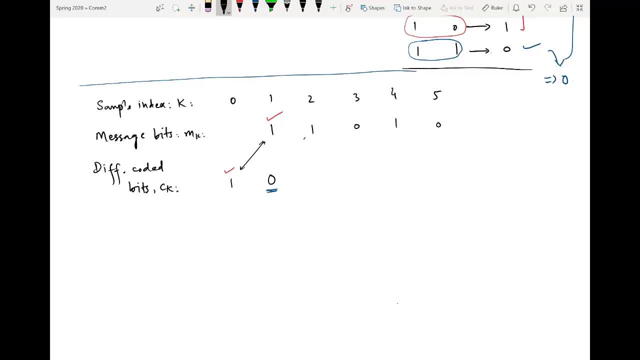 Similarly, XOR of this one will have 1.. Then XOR of this one, we will have 1.. Then XOR of this one, we will have 0. And then XOR of this one, we will have 0.. So in this way the coded bits are formulated. 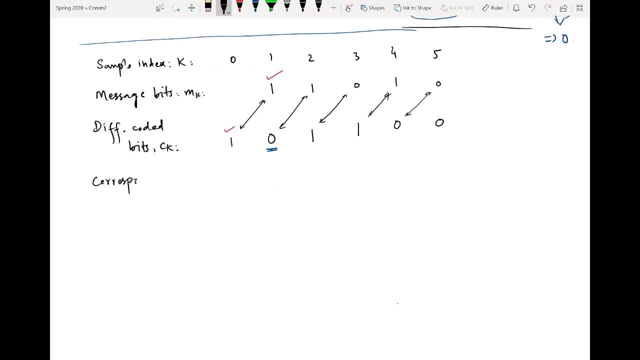 Now the corresponding phase shift because we are talking about binary. So in case of binary we only have two phases: One is pi and the other one is 0. So corresponding phase: theta K. What is that phase? The phase will be assigned by just looking at the coded bit. 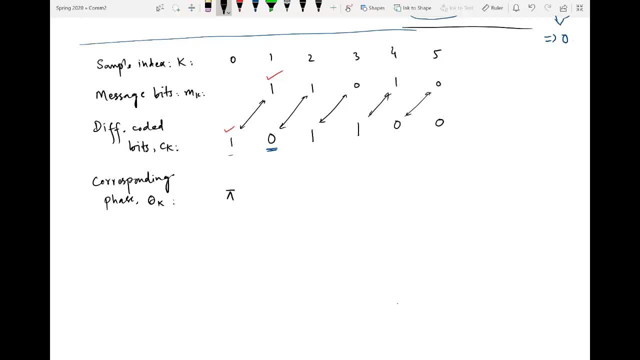 If the coded bit is 1, we will say that the phase is pi. If the coded bit is 0, we will say that the phase is 0. So, correspondingly, all these phases will be allocated. Now, you see, while allocating the phase, we have not seen the previous bit. 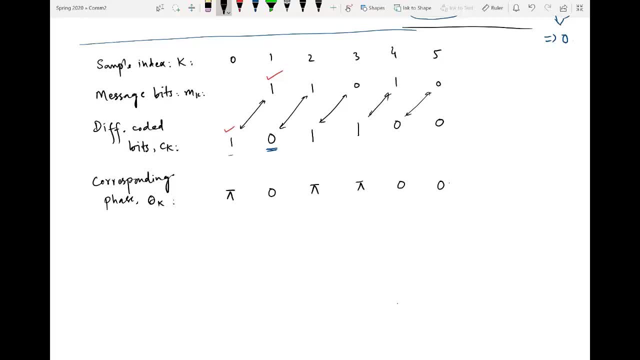 because already we have differentially encoded the data. We are not assigning this phase By looking at MK, we are assigning these phases by looking at CK, And CK is already differentially encoded. So this is how you formulate the corresponding phase shift in the binary DPSK scheme. 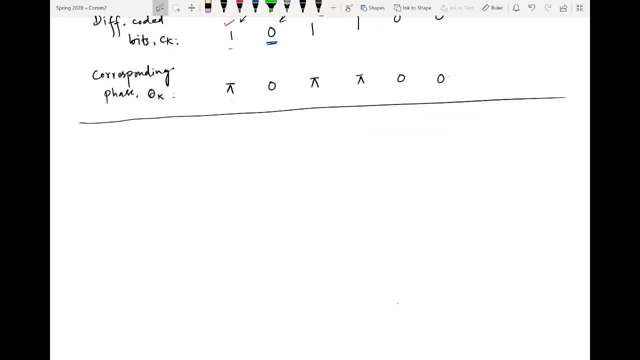 So this is the transmitter side. Now, if you look on the receiver side, On the receiver side, what we need to do, Because the essence of differential encoding was we need to demodulate the symbol by using not the absolute value of the carrier. 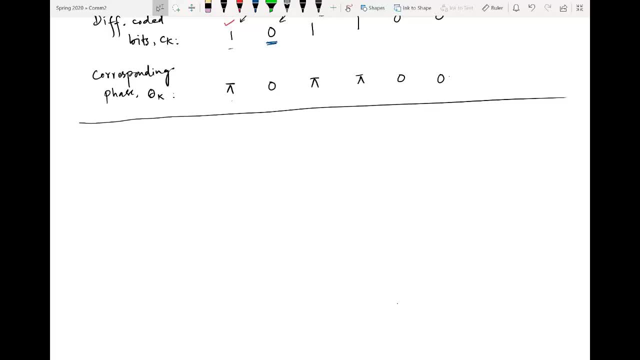 but now the previous symbol or the previous phase will act as the reference. So the decoder will be the same as in case of coherent detection, but there is only difference. So now how the receiver will be working. Remember, we need to make a non coherent detector. 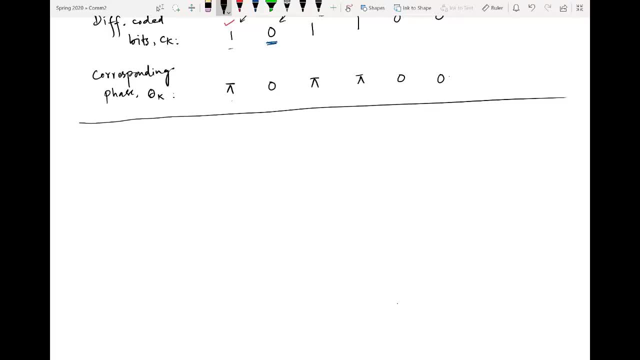 So what is the difference between the coherent and non coherent in this particular scheme? First of all, let me let me draw here the coherent PSK scheme- Coherent PSK detector- And then we will see what is the difference between coherent and non coherent in this particular case. 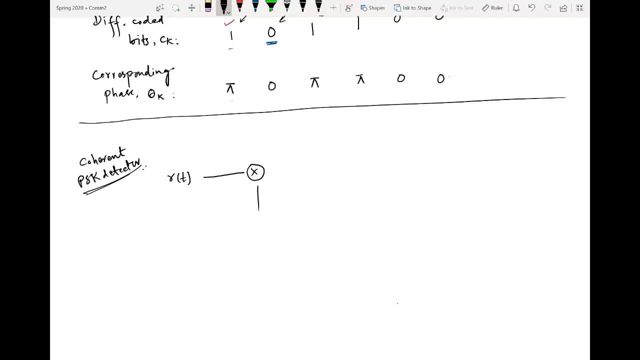 So for coherent. we have a received signal, we multiply it with a locally so for coherent. so for coherent- and detector. the received signal is being multiplied with the basis function, psi 1 of T, and then we have correlated correlator stage from 0 to capital T and followed by decision stage. followed by decision stage to 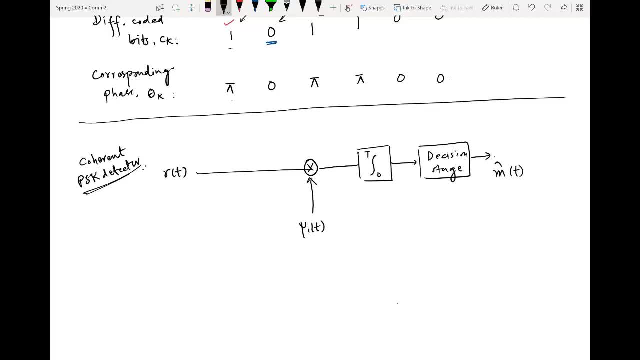 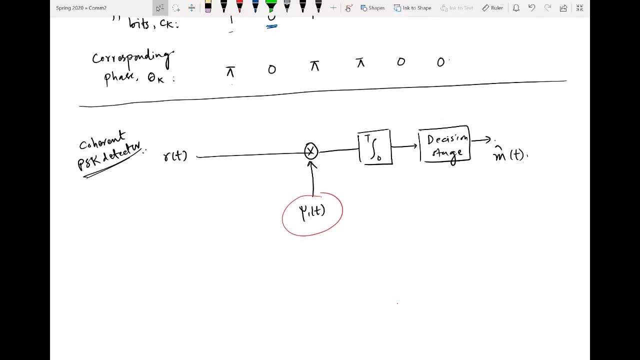 detect M, hat of T. so this is the coherent detector which uses basis function, which makes it coherent because we are using the absolute value of the phase. but now, in this particular case, the only difference will be that, instead of using this basis function, we will be using the previous symbol as the reference, and that will be. 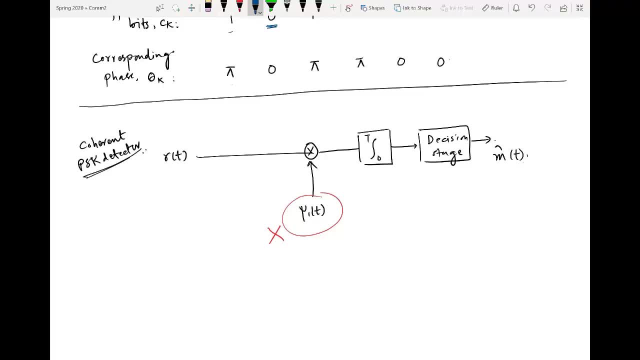 multiplied in the correlation stage. so we will remove this one from here and instead of using this one, we simply use the previous phase, we delay it by capital T and we use it the previous phase, which is acting as the reference over here. so the current symbol and the previous symbol. 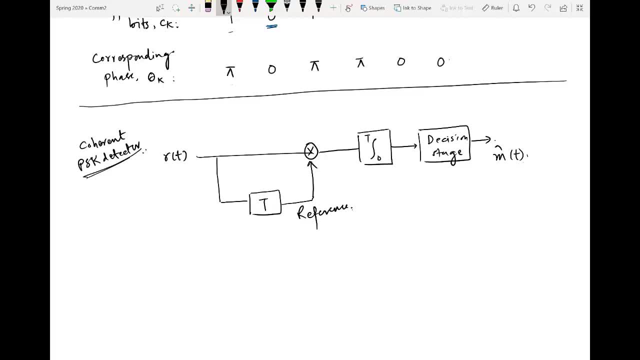 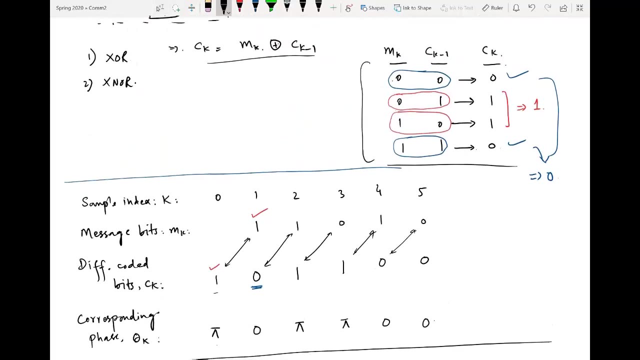 they will become compared if the current and the previous phase are equal. now you see, now the rule of thumb comes over here. if the current phase and the previous phase they are equal, it means that the detected symbol will be 0, as per this truth table. so let 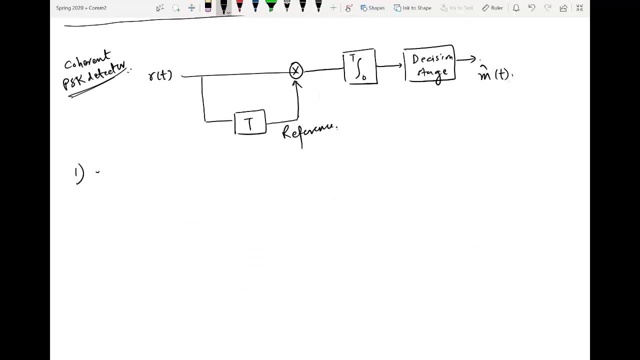 me write these two rules over here. first point will be: if the current and previous phase are equal, it means in that case you will get the maximum correlation out of them and the detected- detected bit will be 0. and if the current and previous phase are opposite or opposite, 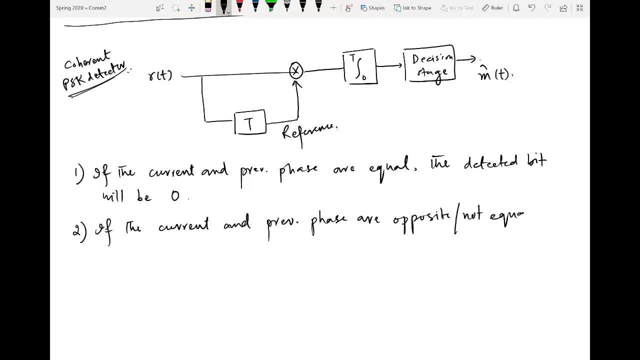 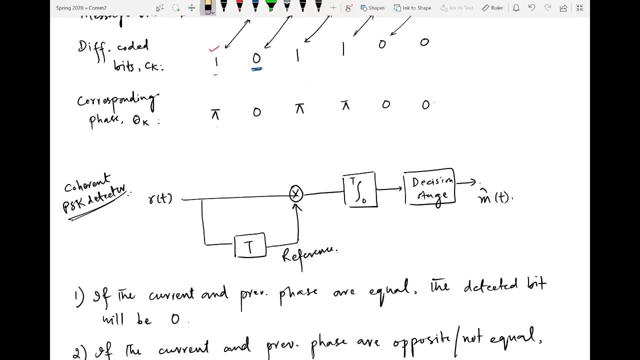 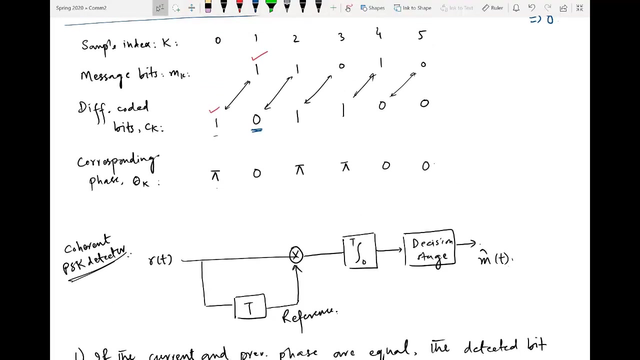 or not, equal detected bit will be 1. now how this case proceeds in this particular diagram. we remove this line from here and you will simply compare the current phase with the previous phase. so here, for K is equal to 1. this is for K is equal to 1 and. 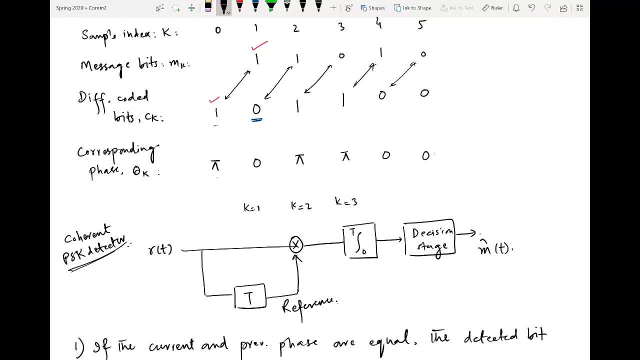 k is equal to 2, k is equal to 3, k is equal to 4 and k is equal to 5.. So at k is equal to 1, the phase is 0 and the previous phase was pi. So they are not equal When they are. 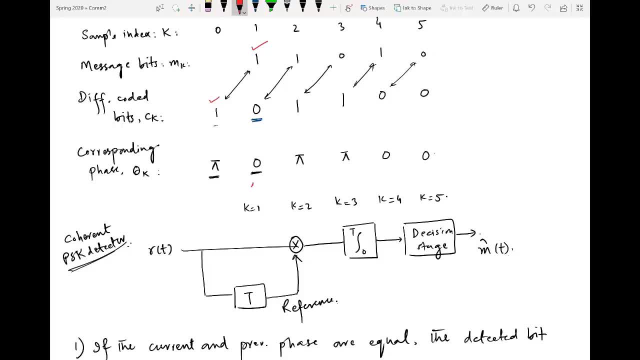 not equal. it means the detected bit will be 1.. So now this row is representing the detected bits m of k in red. So the detected bit will be 1.. Similarly, the next one here for k is equal to 2, the current one is pi and the previous one is 0.. So again, they are different and 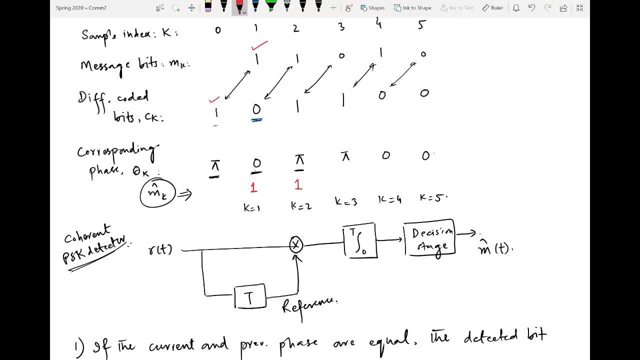 when they are different, as per the decided rule, the detected bit will be 1.. Similarly, for k is equal to 3, k is equal to 3, we have pi and the previous symbol was also pi. It means they are same and when they are same, the detected bit will be 0. 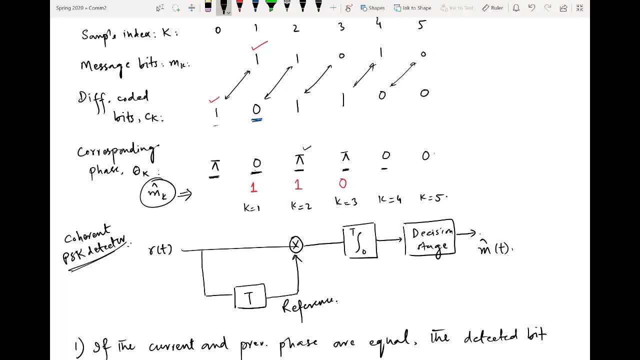 As per the decided rule. Similarly, for the next one, we have phase 0.. The previous one is pi. They are different. So therefore detected bit will be 1 and for the last one, k is equal to 5.. The current bit, the current phase, is 0.. The previous phase was 0.. They are same. 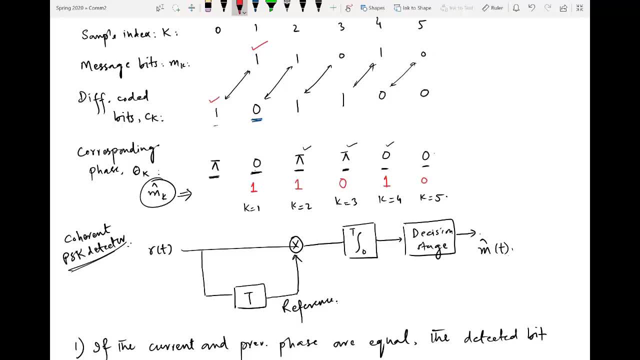 and when they are same, the detected bit will be 0.. Now if you compare these 5 bits with these 5 transmitted bits, directly the transmitted bits were this one, So you can see that the 3 are the same where we have used differential encoding process for performing demodulation. 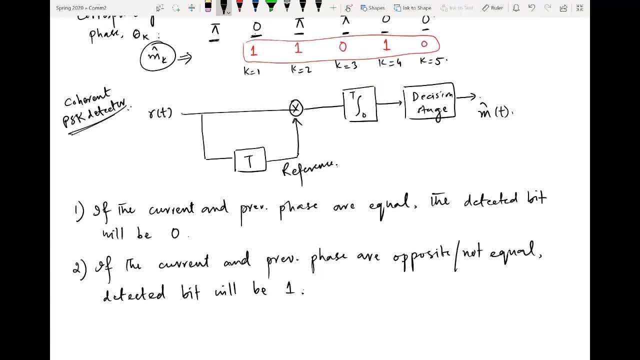 So the same concept can be understood by this particular diagram: that since the previous phase is acting as the reference, so whenever the reference phase is equal to the current phase, it means maximum correlation will be obtained. and in terms of maximum correlation, we will be deciding that to be 1.. 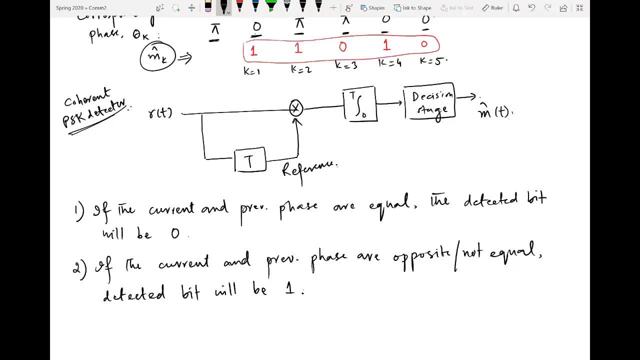 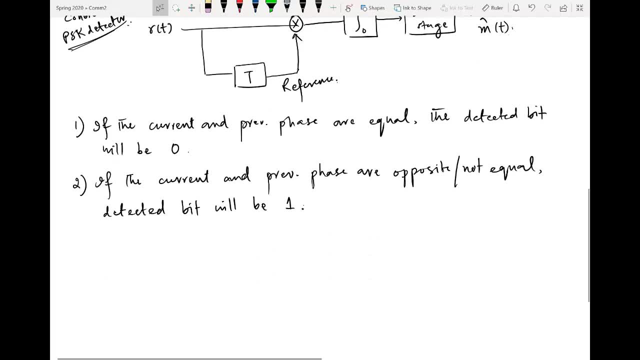 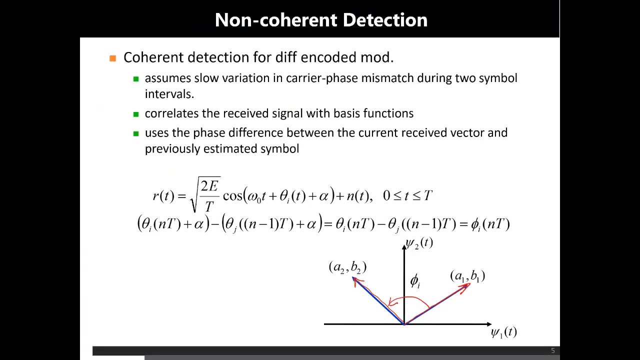 And if they are different, And in that case the detected bit will be 0 because the correlation will be minimum. So in this way we can perform demodulation for differential phase shift keying. But the detector which we have just discussed is basically a sub optimal detector, which 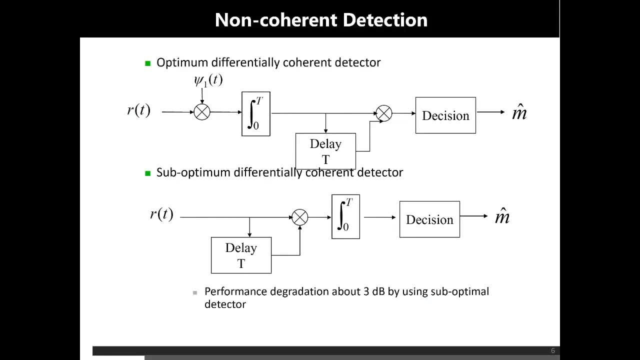 performs the delay prior to correlation. There is an optimal detector for differential phase shift keying in which we first multiply it. We multiply the received signal with psi 1 of t and then correlate, and then after that, after correlation, we perform the delay and then perform the decision. 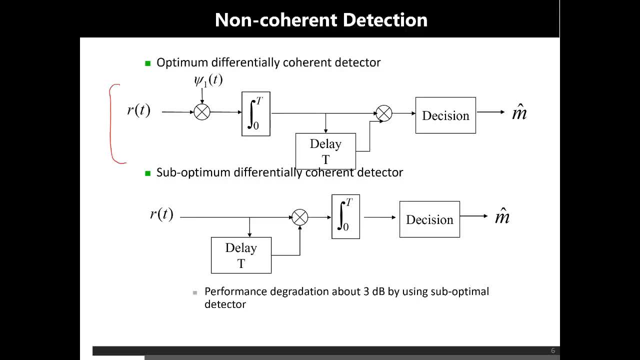 This one. So I am talking about this particular diagram. So this is basically optimal differential in different optimal differentially coherent detector. Why this is optimal? because it is using coherent detector and the performance of coherent detector is always superior to the non coherent detector. and this is coherent because it is using this. 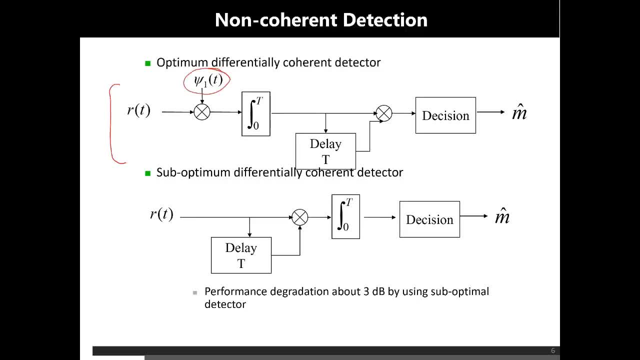 basis function, Exactly the absolute value of basis function in the demodulation process. So definitely the performance of this optimal detector will be better than the suboptimal detector which is not using the reference carrier in the form of absolute basis function. So you can say as a conclusion that although differential phase shift keying supports non 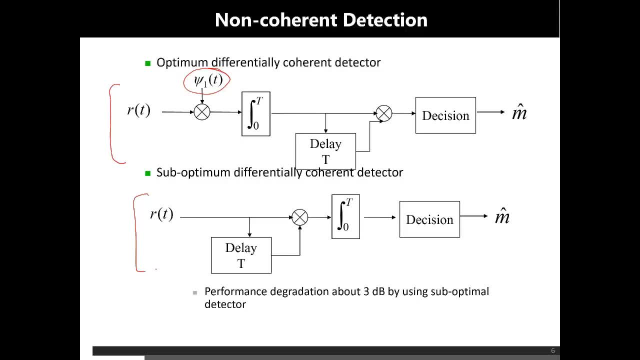 coherent detection. but in order to have better performance out of differential phase shift keying, you can always go for optimal coherent detector shown by the first diagram. But in fact, if you cannot afford coherent detector due to some complexity issues, you can always go for non coherent detection, which will definitely demodulate the data, but it will. it will result. 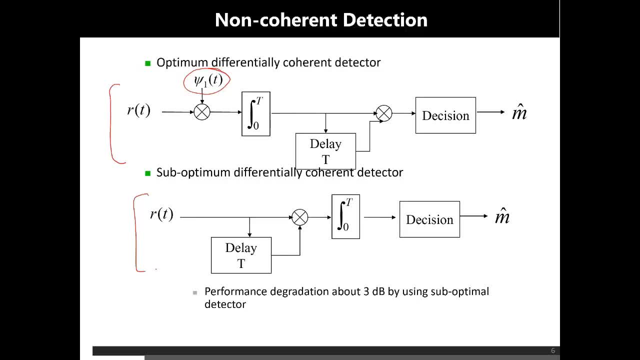 in higher bit error rate as compared to the optimal detector. So that's all for differential phase shift keying. Thank you for watching.